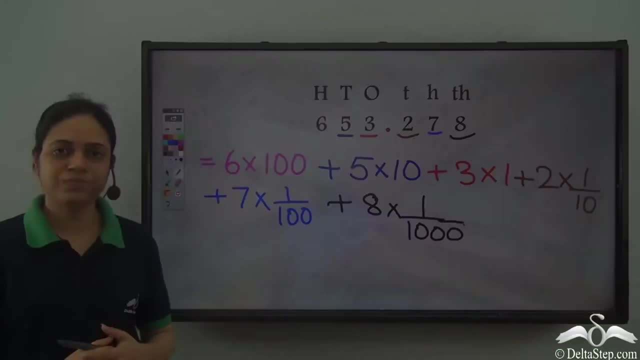 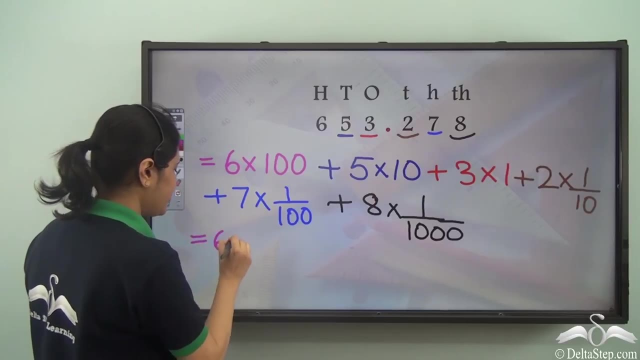 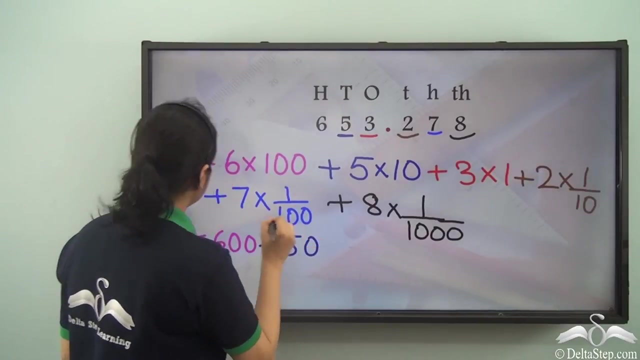 So this is how I can expand this number. Now, another way of expanding. So the way of expanding it is writing it as 6 into 100, as 600.. 5 into 10, as 50.. 3 into 1, as 3.. 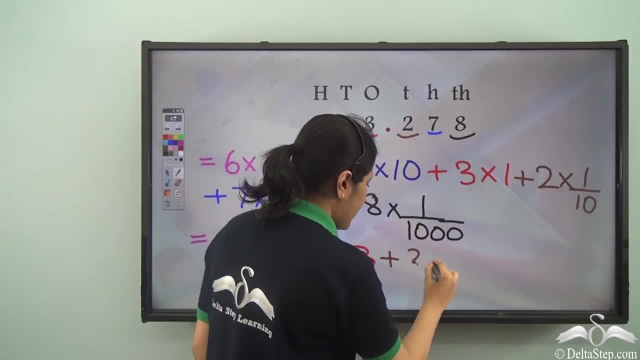 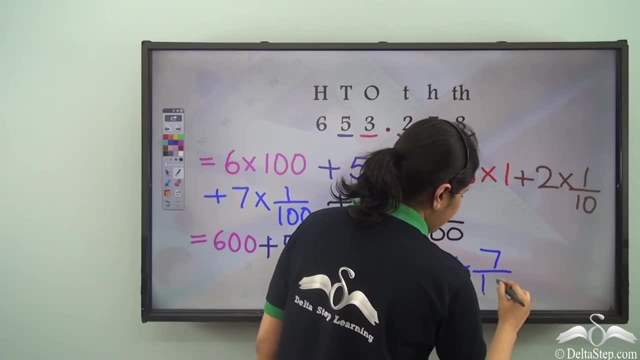 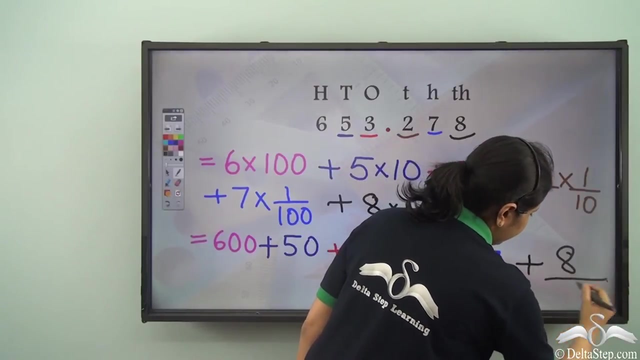 2 into 1 by 10 as 2 by 10.. 7 into 1 by 100 as 7 by 100.. And 8 into 1 by 1000 as 8 by 1000.. So this is how I can expand this number. 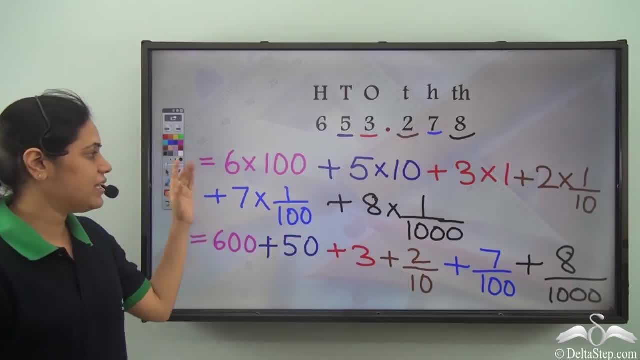 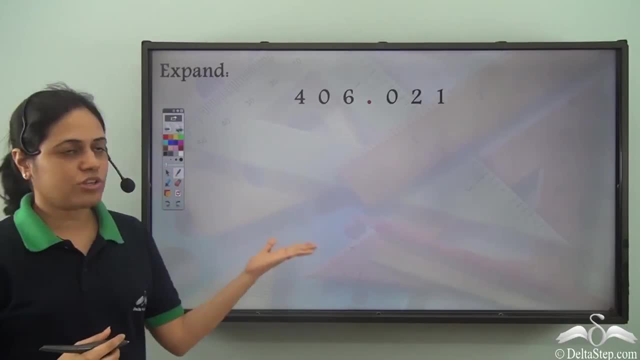 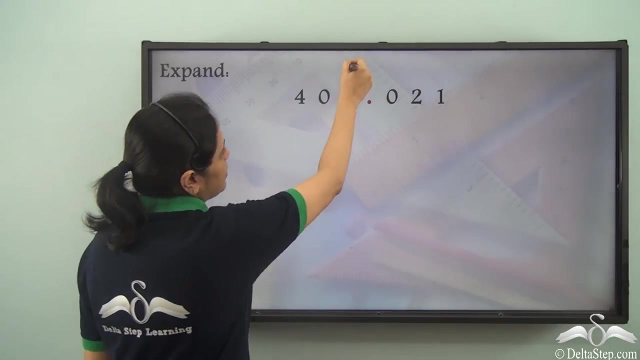 This is how I can expand any decimal number, So I can either expand it like this or I can expand it like this. So now can you expand this number? So, as we can see, this is the 1's place, This is the 10's place. 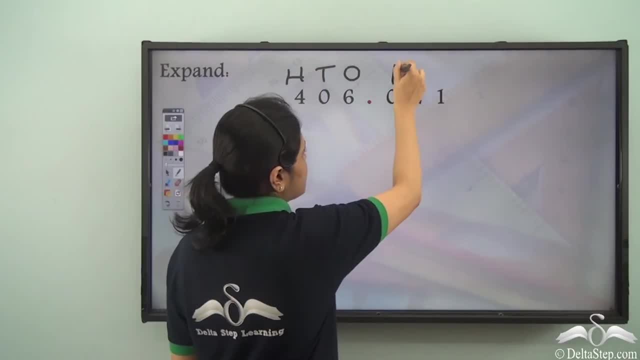 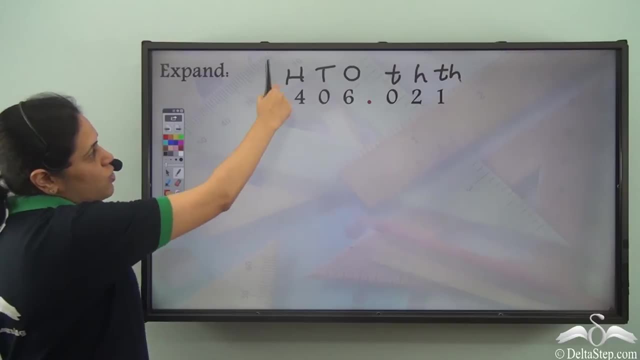 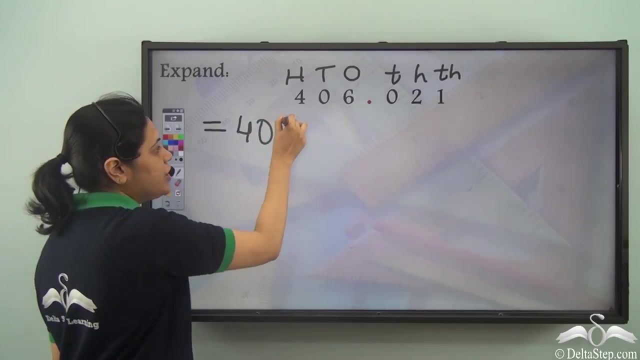 This is the 100's place, This is 10's place, This is 100's place And this is 1000's place. So I have 4 100's, So I can write it as 400.. Then there are 0- 10's. 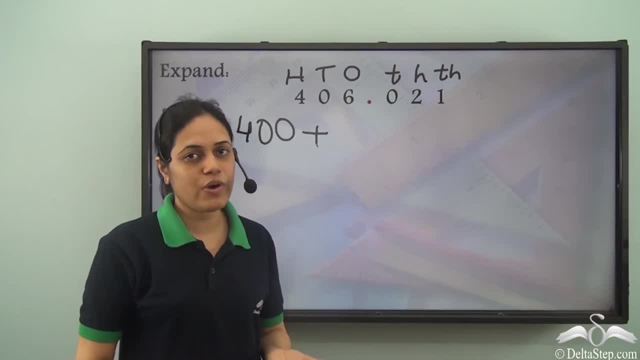 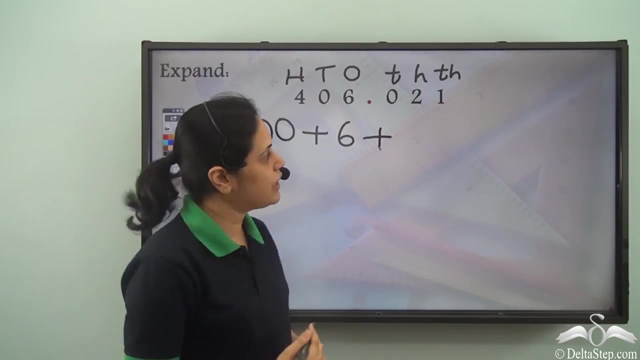 Now adding 0- 10's or we add 0 into anything Means I am adding nothing, So I can ignore this. There are 6- 1's, So this is 6 plus 0- 10's, So once again there is nothing. 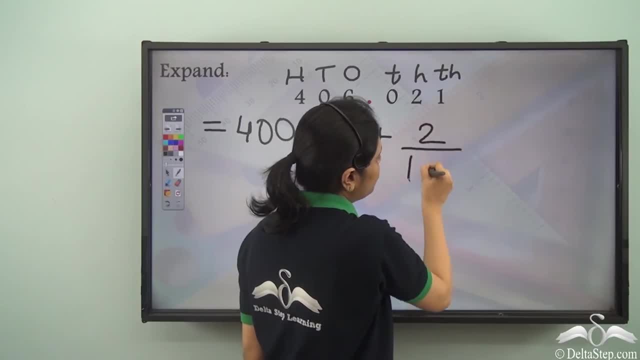 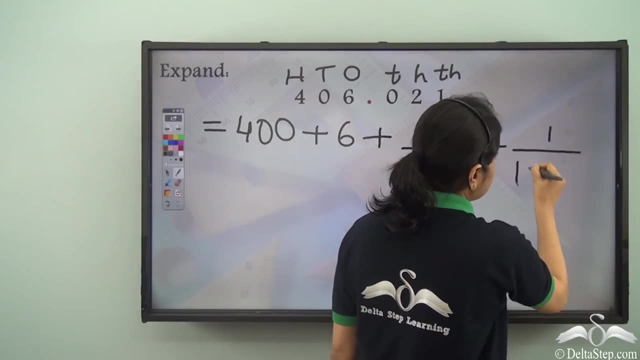 2 100's, So I can write it as 2 100's And 1 1000's, So 1 1000's. So this is how I can expand this number. Now I can expand this number. 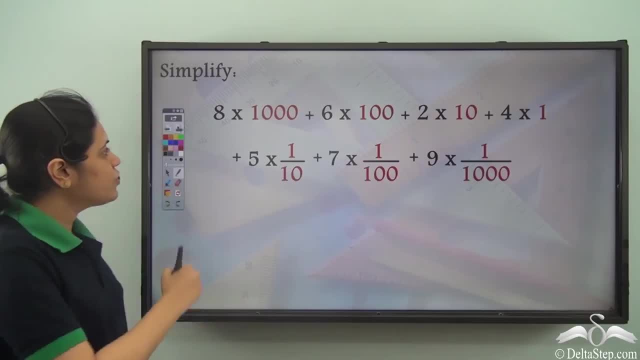 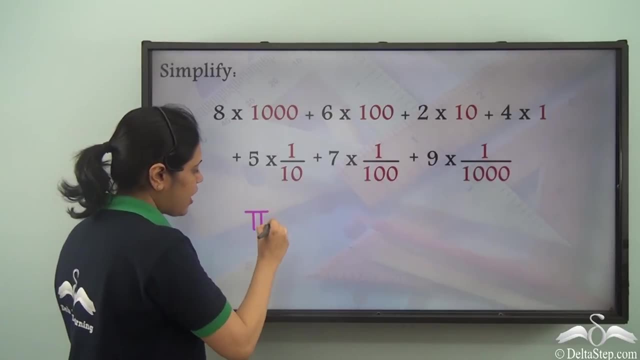 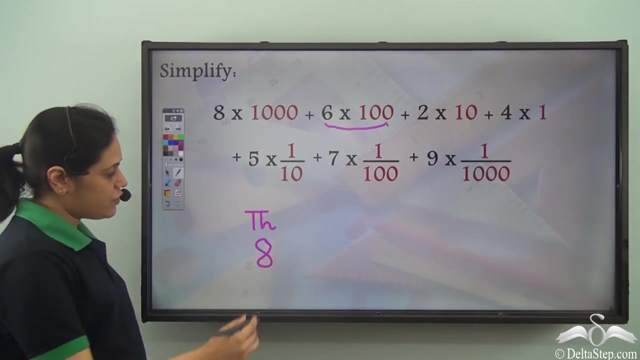 Now can you simplify this number? So we have 8 into 1000. Which means that in the 1000's place there is 8.. Then we have 6 into 100. Which means that in the 100's place 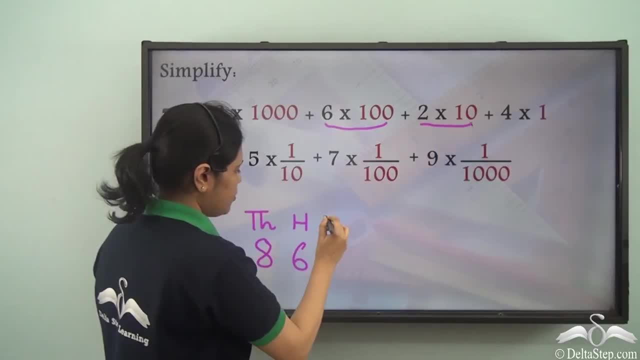 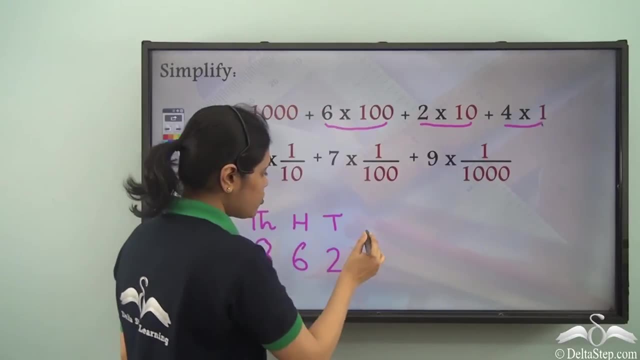 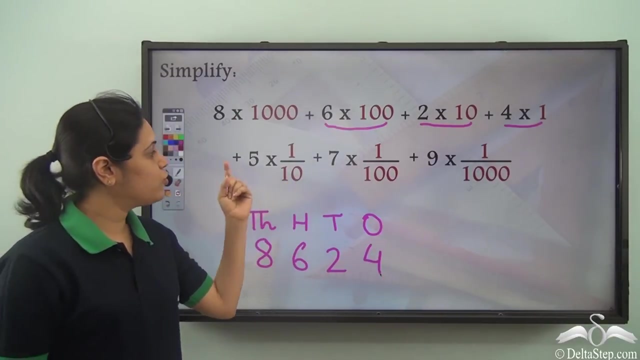 there is 6. Then 2 into 10. So in the 10's place we have 2.. Then there is 4 into 1.. So in the 1's place there is 4.. And then we come to 5 into 1 by 10.. 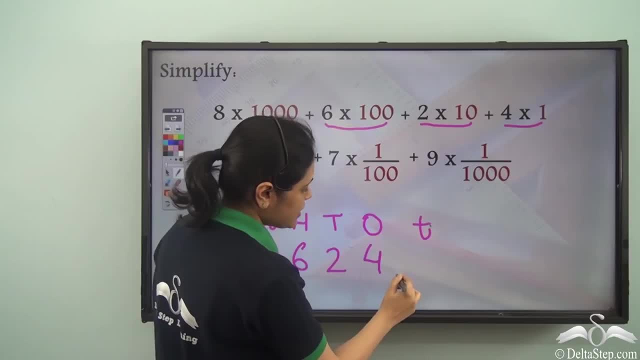 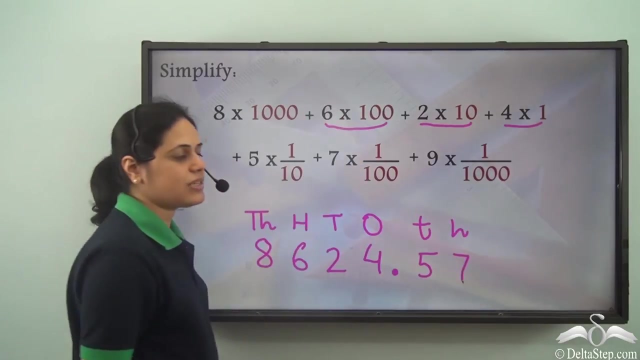 So the 10's place. But after the 1's place I need to put the decimal point And 5 into 1 by 10.. So in the 10's place I have 5.. 5, 7 into 1 by 100.. So in the hundreds place there is 7 and in the thousands place we have 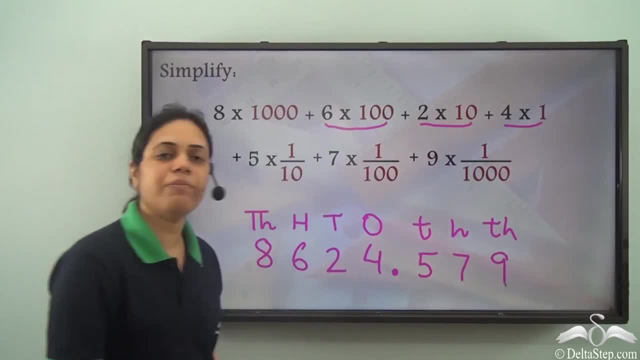 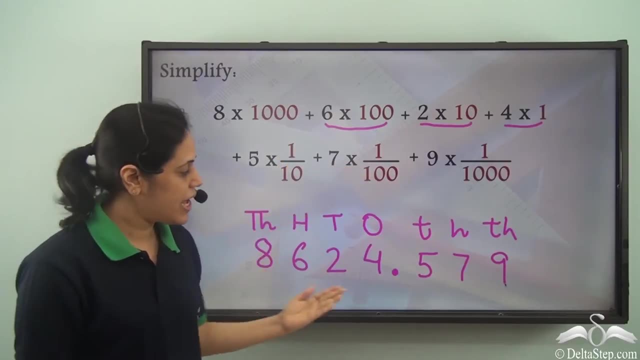 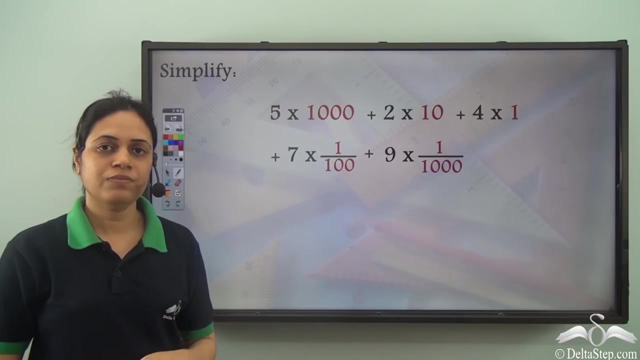 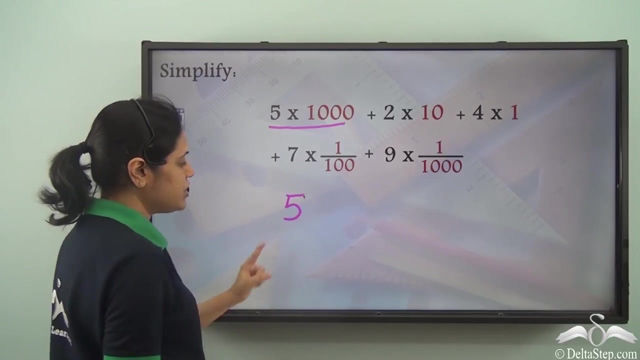 9, because it is 9 into 1 by 1000. So this is the simplified form of this number. So this is the expanded form and this is the simplified form. So now can you simplify this on your own? Let us see: So we have 5 into 1000.. So 5 thousands. Next will be hundreds. 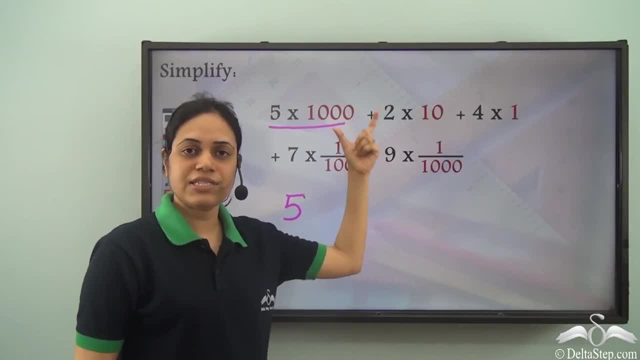 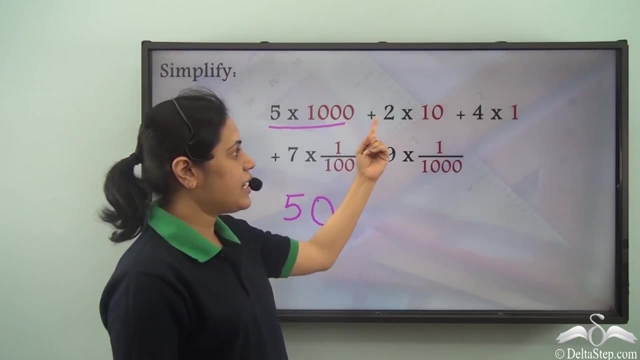 place. But I see that there is no hundreds, Nothing into 100 is given, which means that hundreds place is 0. And then 2 into 10. So there is 2 in the tens place, 4 into 1. So 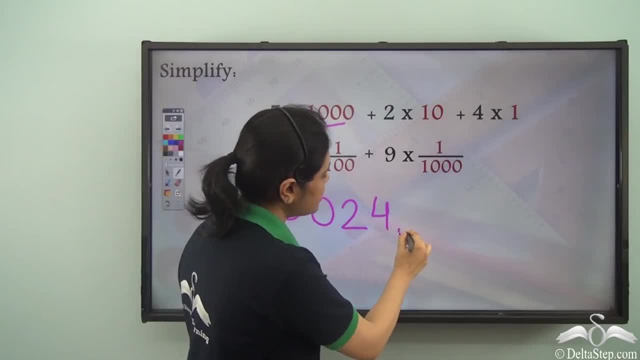 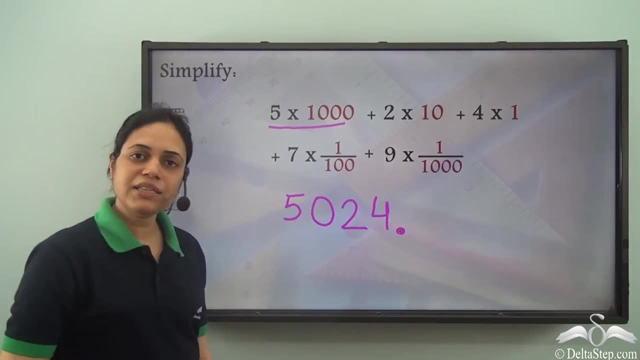 4 in the ones place. After the ones place I need to put a decimal point. Then after the decimal point there should be tens place. I should have something into 1 by 10. But that is missing. So this means that the tens 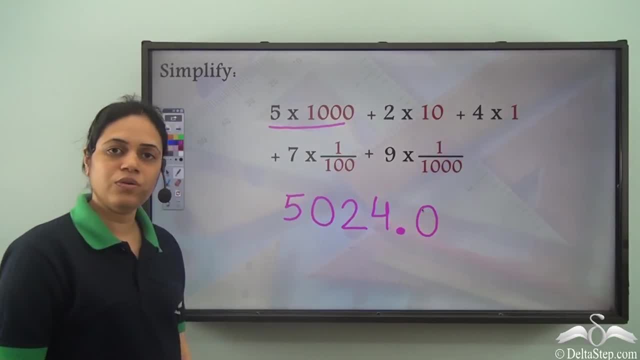 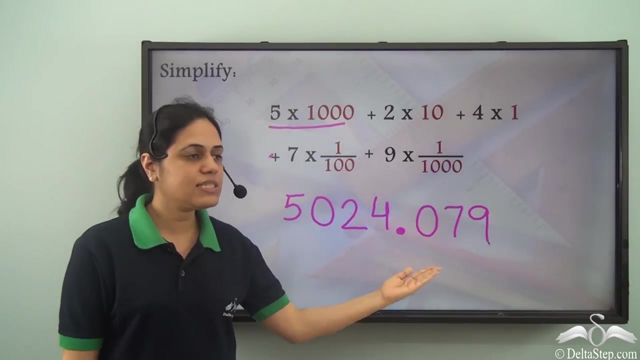 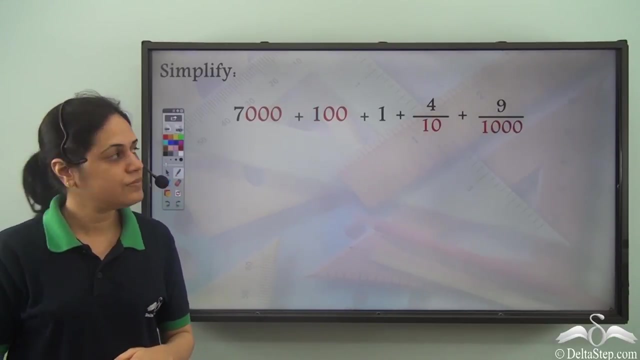 place has nothing or 0. And then in the hundreds place there is 7 and thousands place has 9.. So this is the simplified form of this number: 5024.079.. Now can you simplify this? So there is 7 thousands, So there are. 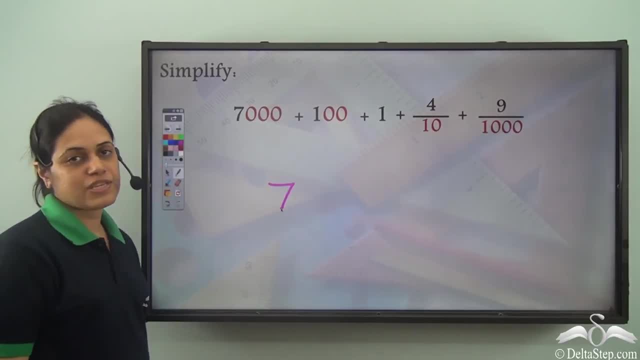 7 thousands. So in the thousands place I have 7. 1 hundred, So in the hundreds place I have 1.. There are no tens, So tens place is 0. 1 ones. So we have 10 here. So in the hundreds.